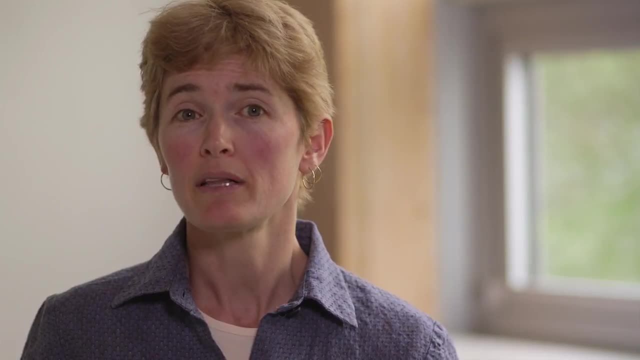 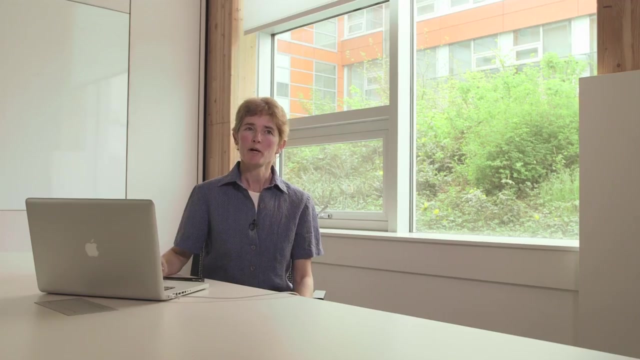 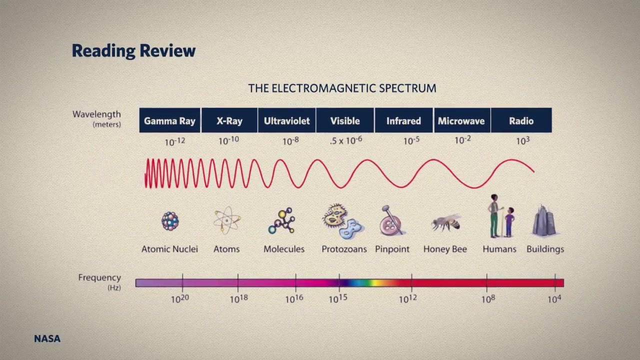 But what we can do is measure characteristics of the electromagnetic radiation coming from the sun and then use physical laws to figure out the sun's temperature. Here's a quick review of the electromagnetic spectrum. Electromagnetic energy comes in different flavors, with different wavelengths, frequencies. 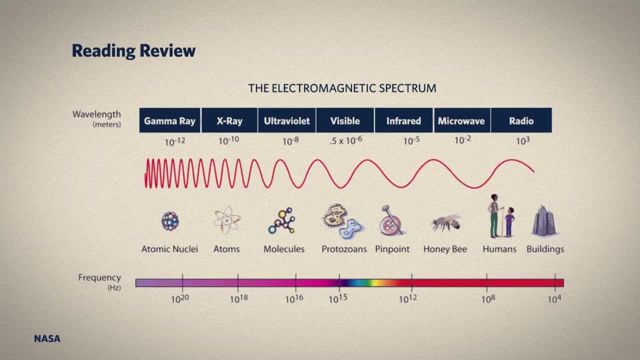 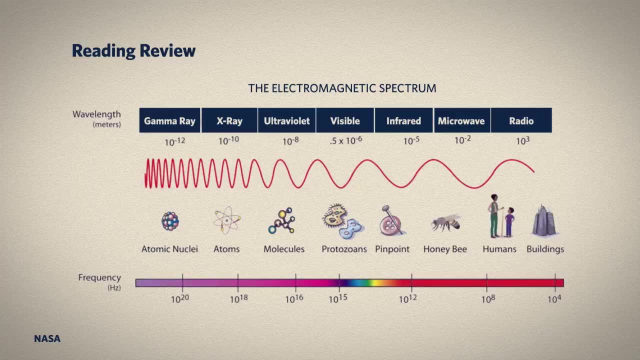 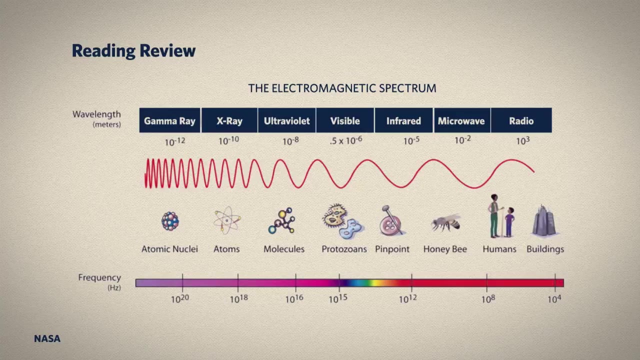 and photon energies. For our purposes, we're primarily interested in wavelengths in the visible range, the infrared and a little bit of ultraviolet. Of these, ultraviolet has the shortest wavelengths, highest frequencies and highest photon energies. You already explored that in a reading. 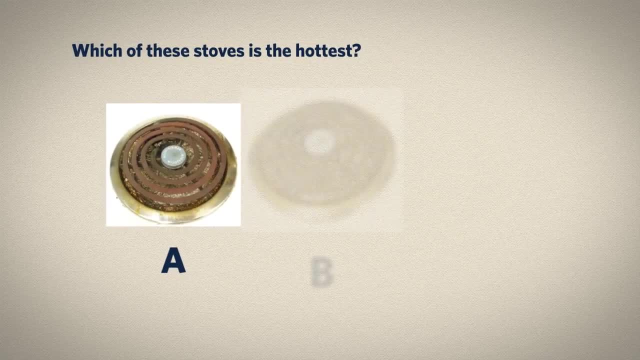 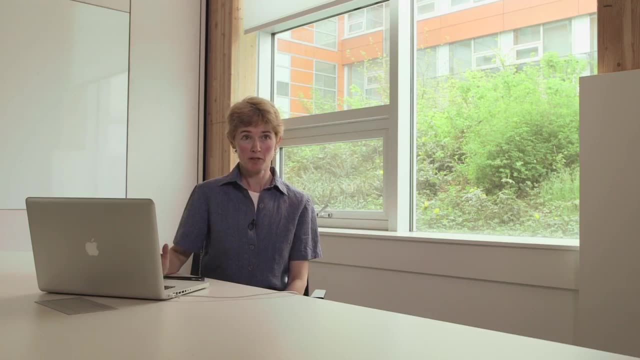 To get warmed up. let's try a couple of questions. Which of these stoves is the sun? Which of these stoves is the hottest? If you said C, you probably have some experience with electric stoves like mine And you know it's probably not a good idea to put your hand down on a red burner, because 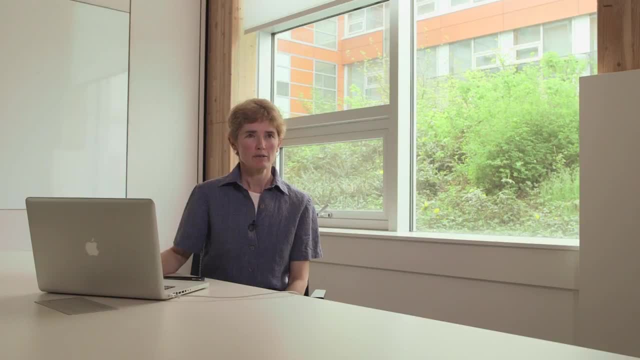 it's hot and it's giving off a lot of energy and you might get burned. A black burner is definitely cooler than a red burner. So there seems to be some relationship between the stove color, the temperature and the amount of energy the stove gives off. 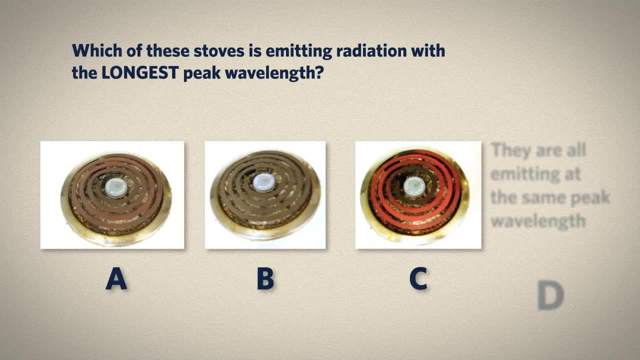 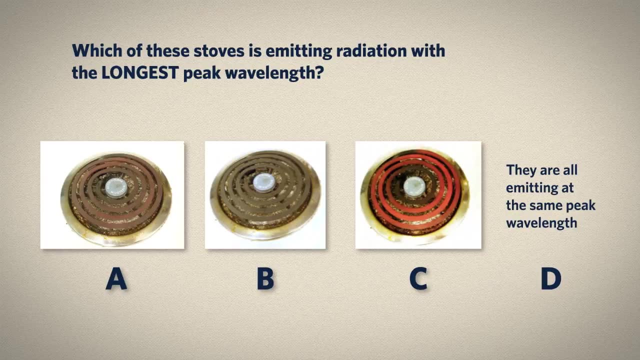 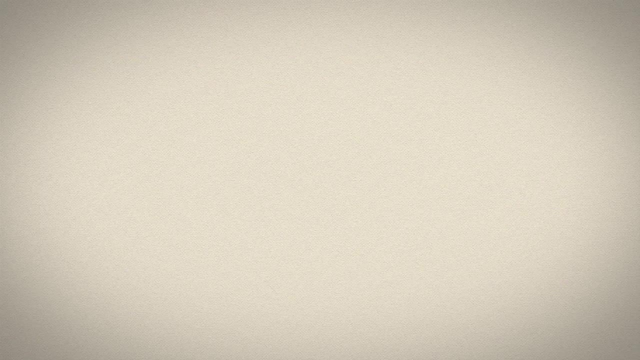 Try this question next. This one's a little harder. Which of these stoves do you think is emitting radiation with the longest peak wavelength? Think about what part of the electromagnetic spectrum would correspond to the emissions of these three stoves. Stove C- we can tell- is red. 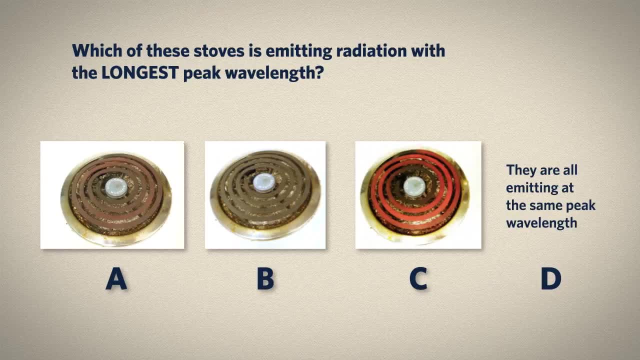 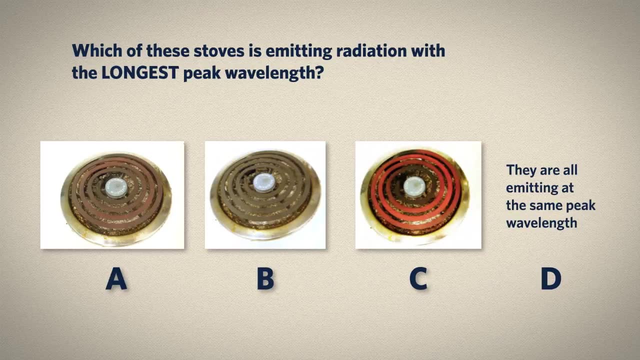 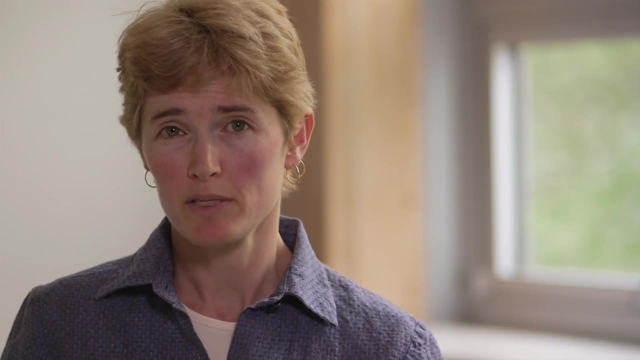 It's emitting some radiation in the visible range which human eyes can see. Stove B, however, is black here in this picture, Which was taken at room temperature. That stove is emitting radiation at wavelengths that we can't see. These wavelengths are in the infrared part of the spectrum, which are longer wavelengths. 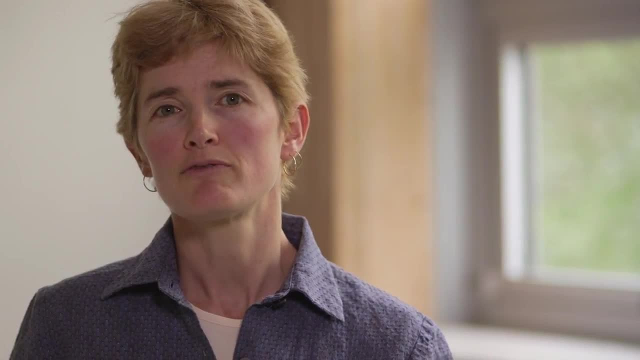 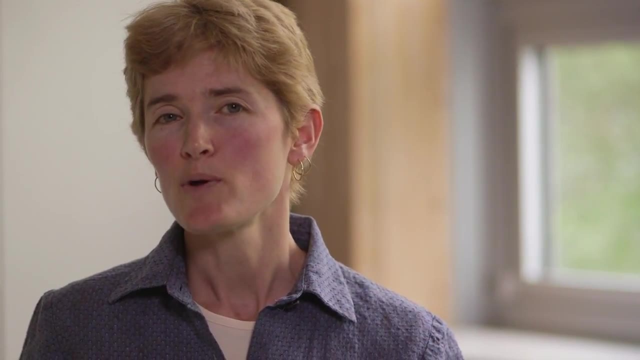 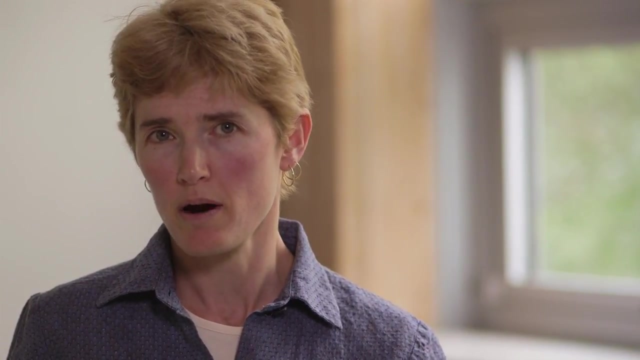 than visible light. Infrared is the same range of radiation that you and I also emit. We're not actually hot enough to emit visible light. If we were able to crank up the temperature on these stoves further, the elements would get brighter and might start emitting light in the yellow part of the visible spectrum. 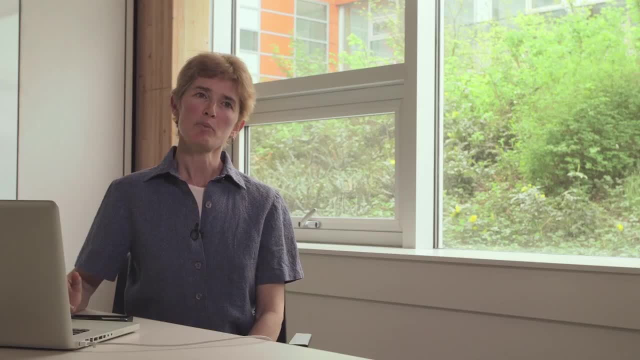 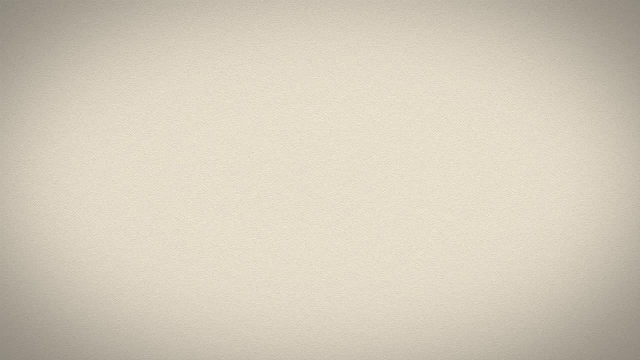 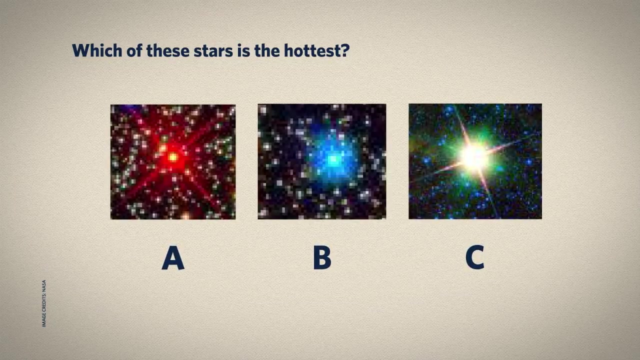 At shorter wavelengths than the red. So let's apply that idea to some stars. Which of these stars is the hottest? Star A looks like it's mostly emitting red light, Star B looks like it's mostly emitting blue light, And star C looks like it's mostly emitting yellow light. 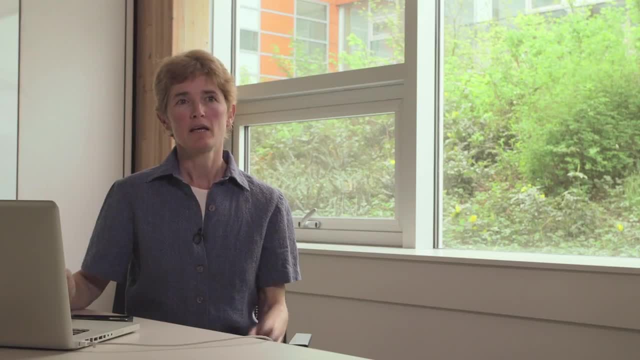 Thinking about the electromagnetic spectrum, red is at the long wavelength end of the visible range, Yellow is in the middle And blue is at the short wavelength end. So, just like the stoves, the star that emits the shortest wavelengths is the hottest. 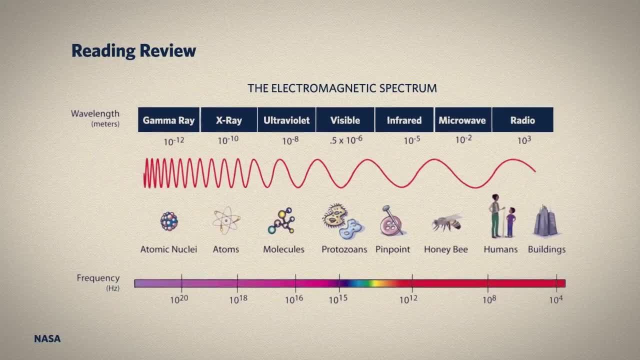 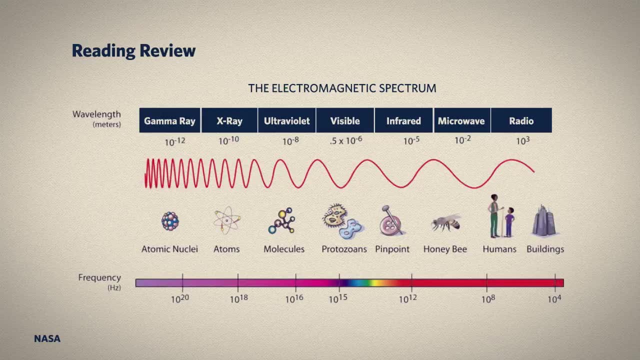 And in this example that's star B. Here's the electromagnetic spectrum again, which can help us see that the blue star emits shorter wavelengths than the red star. So this is pretty cool and we can use it. There's even an equation for it. 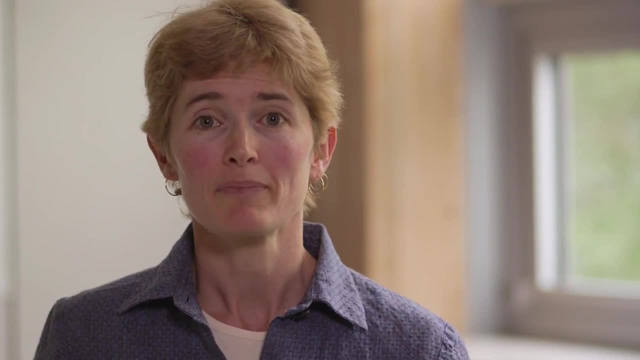 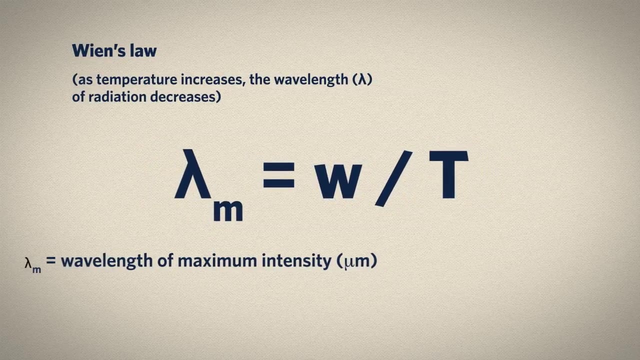 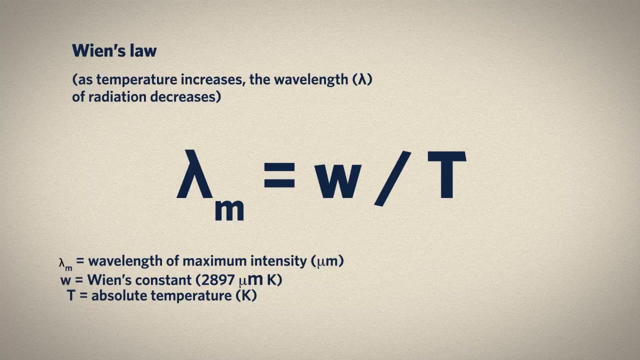 A fairly long time ago, some physicists, notably a person named Wilhelm Wien, Figured out the relationship between an object's temperature and the peak wavelength of radiation that it emits. In the equation here the T stands for temperature, and that's on the Kelvin temperature scale. 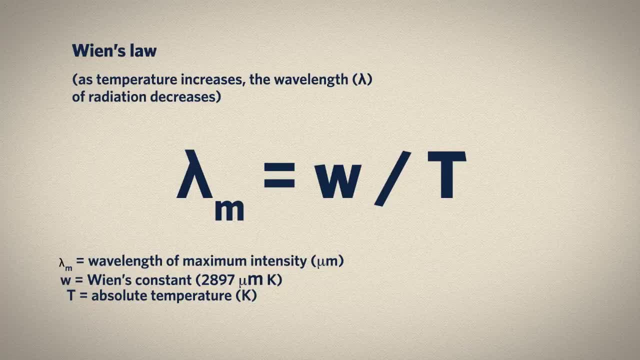 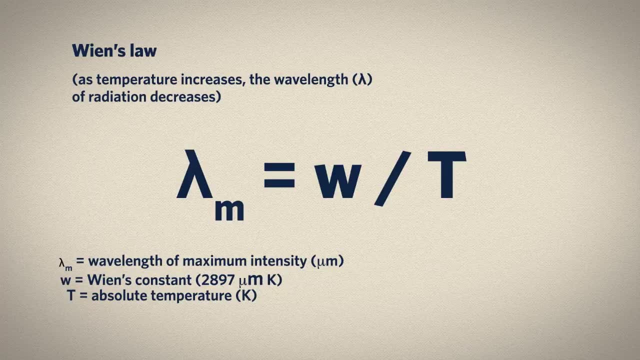 The lambda with the little m next to it stands for the peak wavelength emitted in units of micrometers. And then the W is a constant. that Wien figured out by doing a lot of observations. You might not like equations very much and we won't have very many of them. But this is one that's important. The key thing to note here is that if temperature goes up, the wavelength of maximum emission goes down. Hotter objects emit radiation at shorter wavelengths, just like those stoves and those stars. Getting back to our question about the sun's temperature, this equation lets us figure. 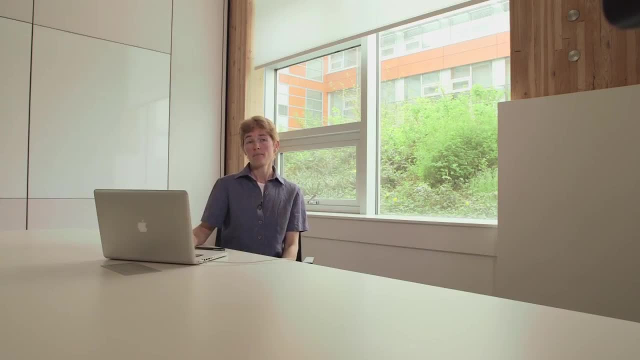 it out. We can save ourselves a trip to the sun by measuring the peak wavelength of the radiation coming off the sun And using Wien's law to calculate the sun's temperature. So we do it: We measure the spectrum of electromagnetic radiation emitted by the sun and we find. 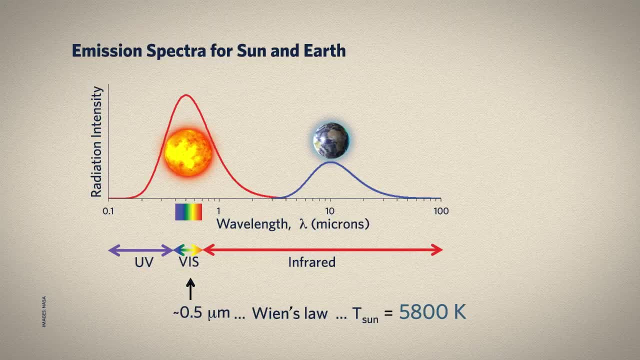 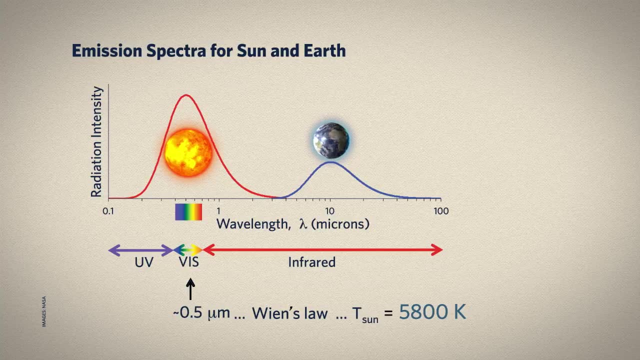 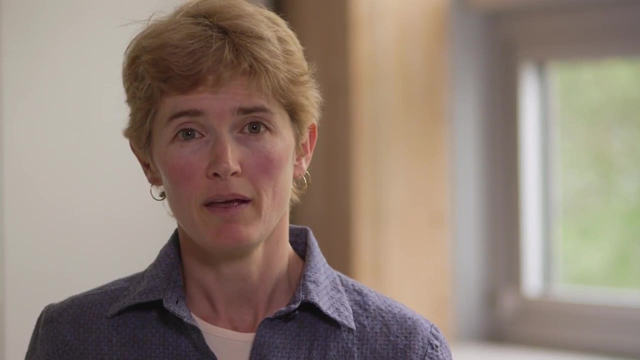 out that the sun's wavelength of maximum emission is in the visible range. Not surprising. you probably knew that. And more specifically, the peak is at about half a micron wavelength. That's the peak or wavelength of maximum emission in Wien's law. 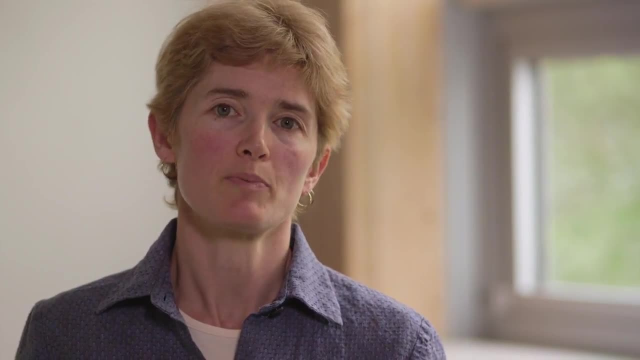 Of course the sun also emits radiation all across the planet, And that's the peak wavelength. It emits radiation all across the visible part of the spectrum And also emits ultraviolet and infrared radiation, but those are on the sloping sides of its emission spectrum. Okay, with a peak wavelength of half a micrometer, we can now use Wien's law and figure out the sun's temperature. After a little algebra, we find out that the sun's temperature is close to 5,800 Kelvin. 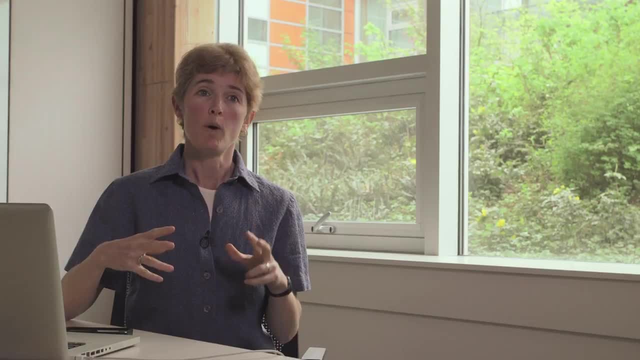 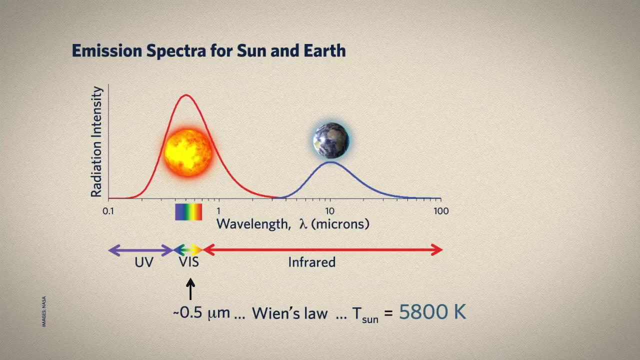 which is pretty hot. So what about Earth? You can see here that the spectrum of radiation Earth emits is 5,800 Kelvin, which is pretty hot, And the temperature that Earth gives off is out in the infrared at longer wavelengths, which is expected, since we know that the Earth is cooler than the sun. 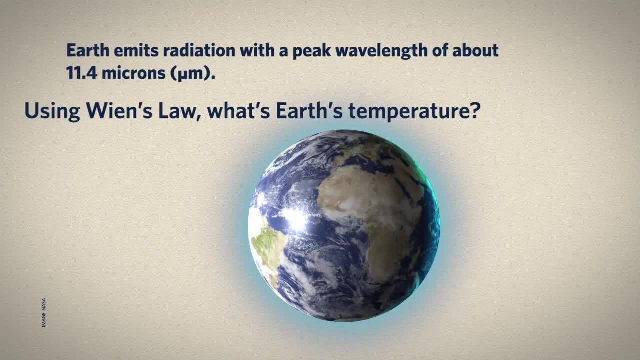 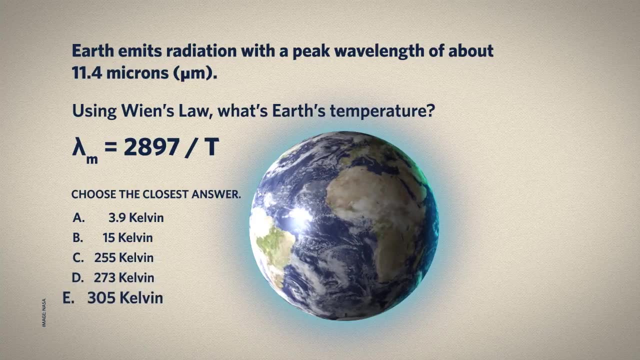 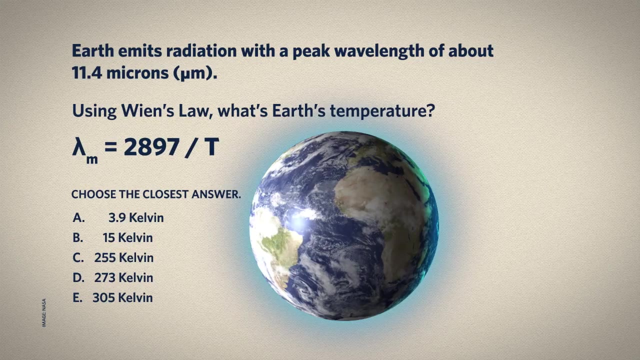 So let's try a question about that. At the top of Earth's atmosphere, the planet emits infrared radiation at a peak wavelength of about 11.4 micrometers. What temperature does that correspond to? From Wien's law, we find out that the temperature at the top of Earth's atmosphere is about: 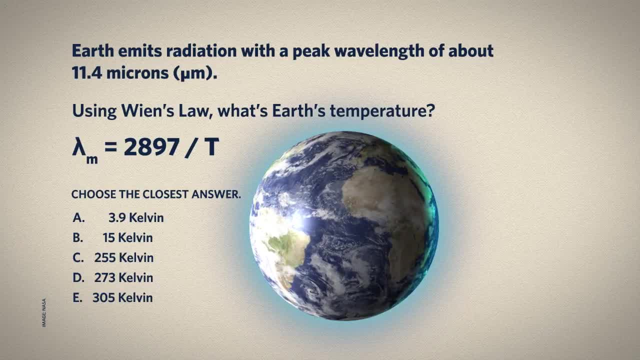 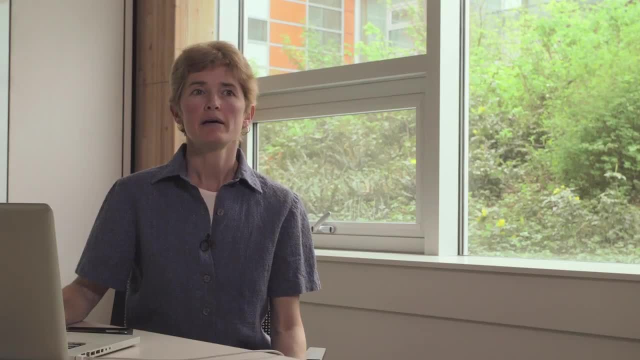 5,800 Kelvin, And the temperature at the bottom of Earth's atmosphere, where energy is radiating to space, is about 255 Kelvin, or choice C here, which is about the same as minus 18 degrees Celsius or about zero degrees Fahrenheit. 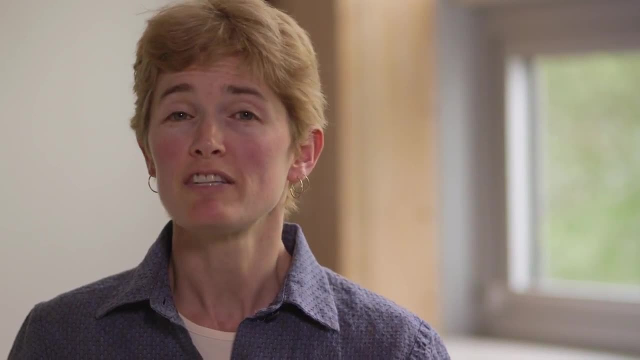 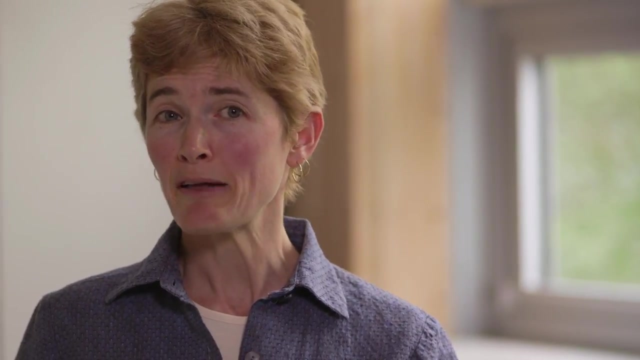 It's pretty cold up there. So we've determined that the sun and Earth give off different types of energy, which is going to become important when we talk about the greenhouse effect, But also, as you can probably imagine, every square meter of the sun's surface emits tremendously. 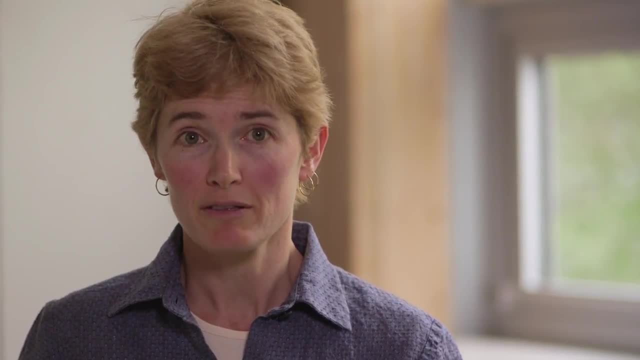 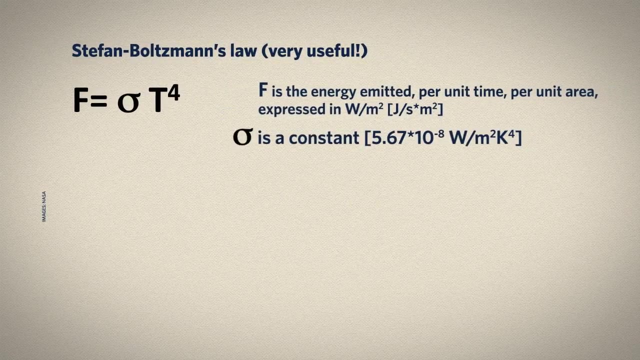 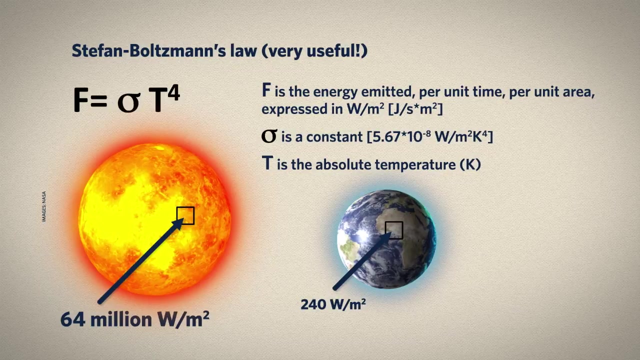 more energy every second than every square meter of Earth emits. This is the other important law relating temperature and energy. This one was figured out by two people, Stefan and Boltzmann, So it's the Stefan-Boltzmann law. This relationship says that as temperature increases, the amount of energy given off. 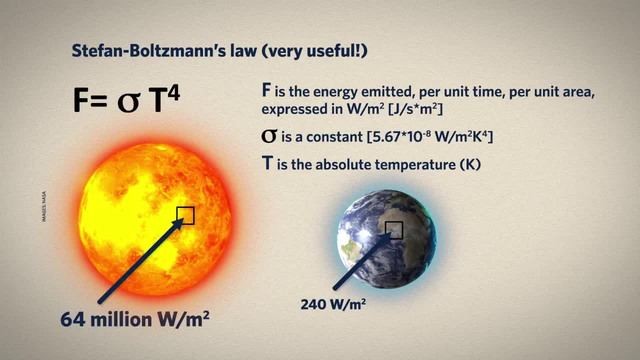 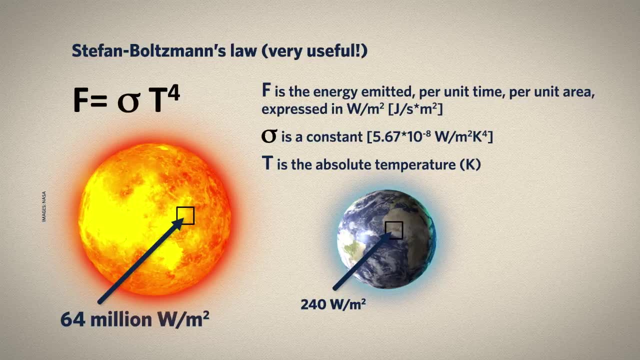 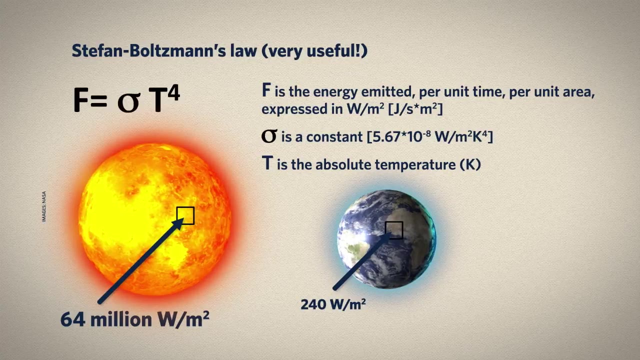 by an object per second per area, goes up exponentially to the fourth power. So, for example, if you double the temperature, the energy given off, the energy given off per second per square meter doesn't just double, It goes up by 16 times. 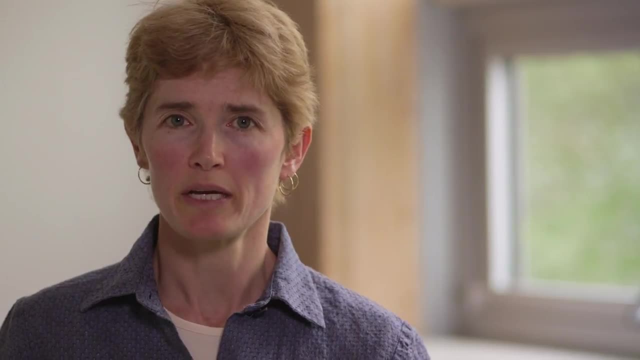 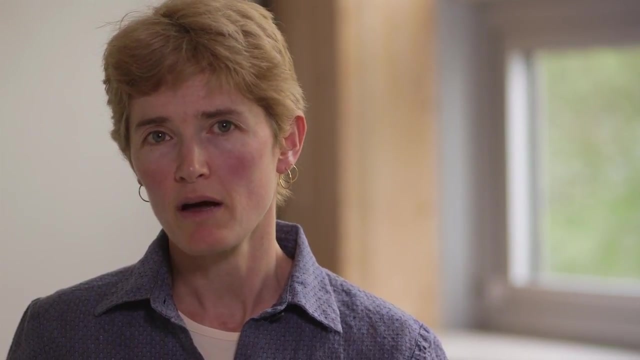 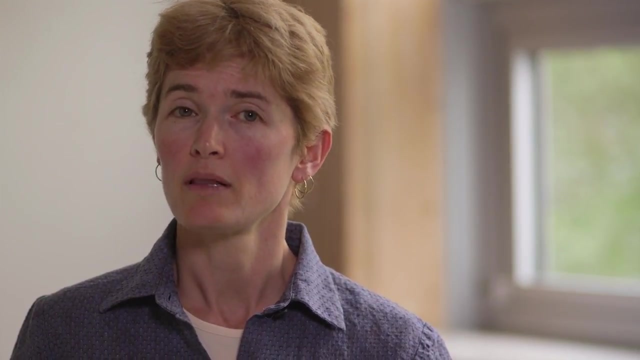 So it goes up a lot. Recall that the energy per photon is higher for shorter wavelength, higher frequency radiation, like ultraviolet radiation, Thinking about Wien's law: as something gets hotter, it emits shorter wavelength radiation which has higher energy per photon. The Stefan-Boltzmann law takes into account that increased energy per photon at shorter wavelengths. Do the math, and I'd encourage you to try the math. We come up with the answer that each square meter of the Sun's surface gives off about. 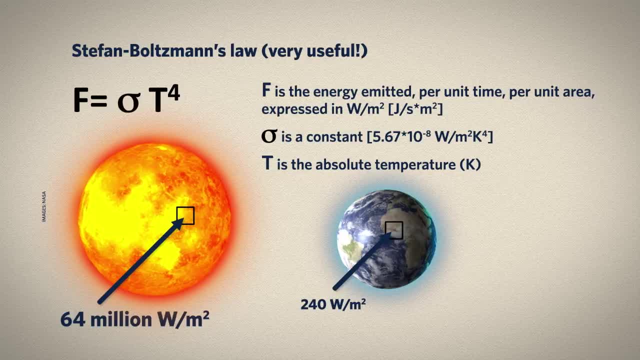 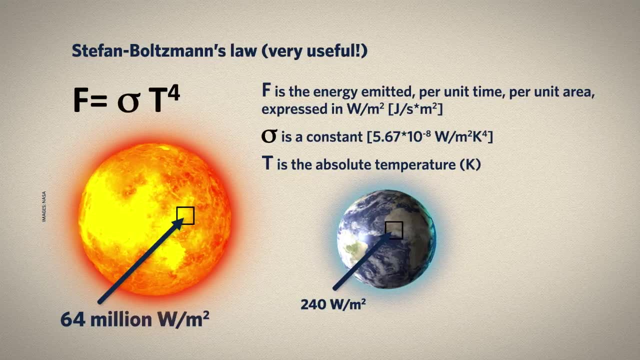 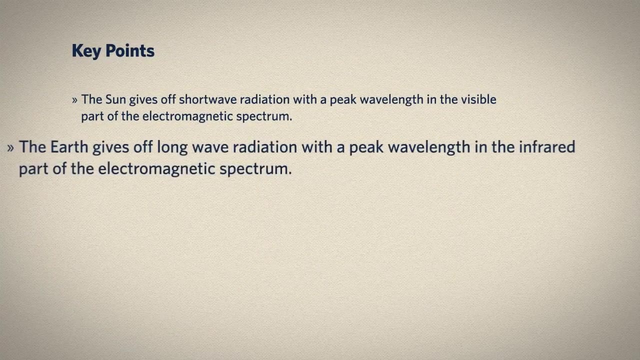 64 million joules every second. In contrast, the Earth's upper atmosphere gives off only about 240 watts per meter squared. Just imagine those boxes drawn on the Sun and the Earth as only one meter square. Alright, key points from this lesson.